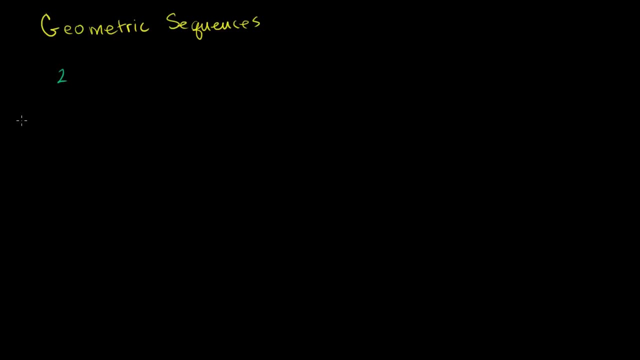 So let's say my first number is 3. And then I multiply 2 by the number 3. So I multiply it by 3,, I get 6.. And then I multiply 6 times the number 3, and I get 18.. 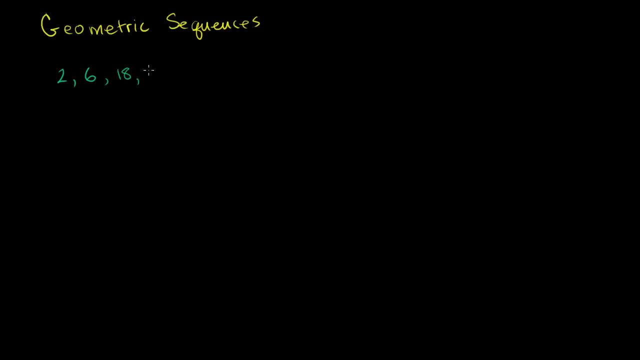 And then I multiply 18 times the number 3, and I get 54. And I just keep going that way. So I just keep multiplying by the number 3.. So I started- if we want to get some notation here- this: 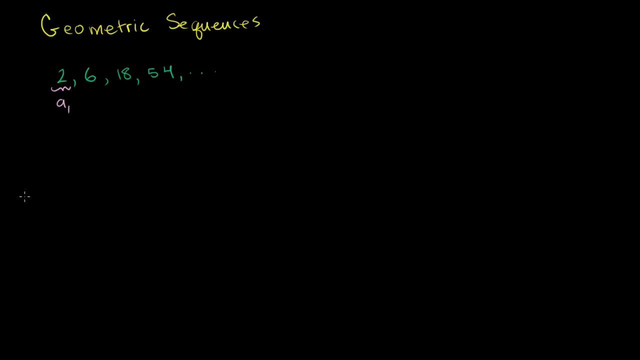 is my first term, We'll call it a1 for my sequence, And each time I'm multiplying it by a common number, And that number is often called the common ratio. So in this case, a1 is equal to 2.. 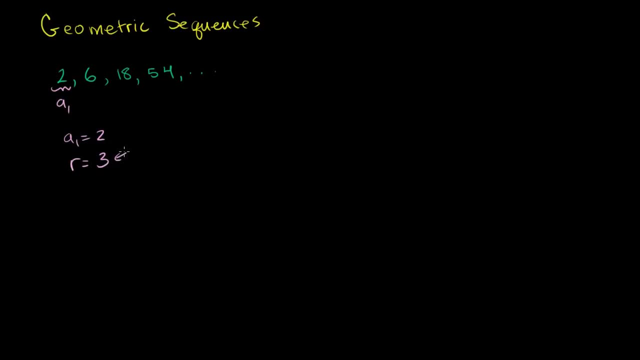 And my common ratio is equal to 3.. Common ratio. So if someone were to tell you: hey, you've got a geometric sequence, a1 is equal to 90, and your common ratio is equal to negative 3.. OK, 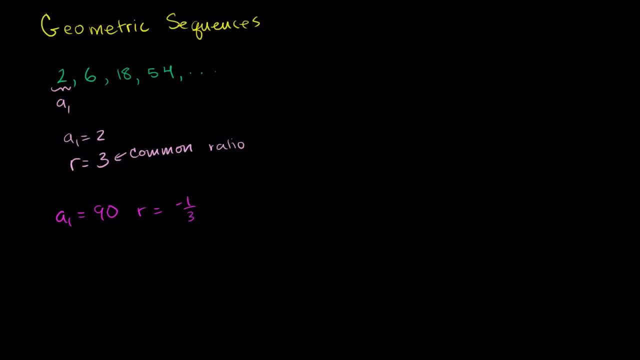 Negative 1 third. That means that the first term of your sequence is 90.. The second term is negative 1 third times 90, which is what That's: negative 30.. 1 third times 90 is 30. And then you put the negative number. 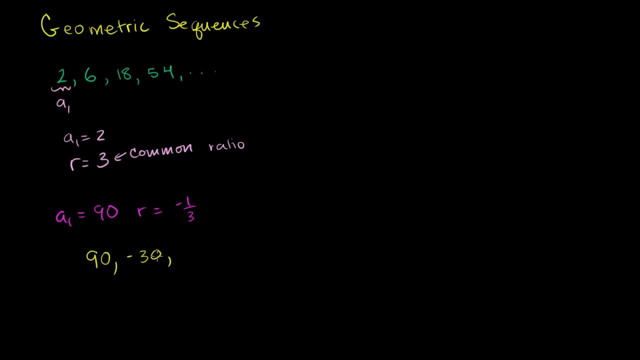 Then the next number is going to be 1 third times this. So 1 third or negative, 1 third times this. 1 third times 30 is 10.. The negatives cancel out, So you get positive, Positive, 10.. 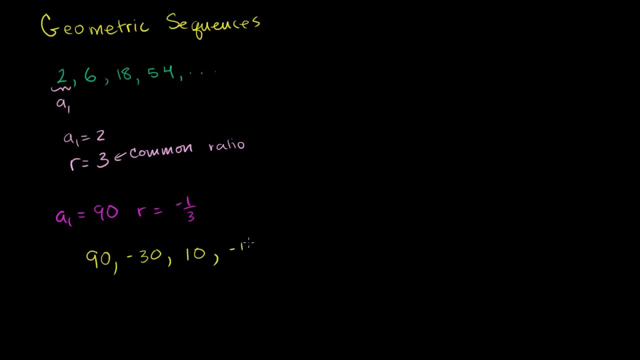 Then the next number is going to be 10 times negative: 1 third, or negative 10 thirds. And then the next number is going to be negative 10 thirds times negative: 1 third. So it's going to be positive 10 thirds. 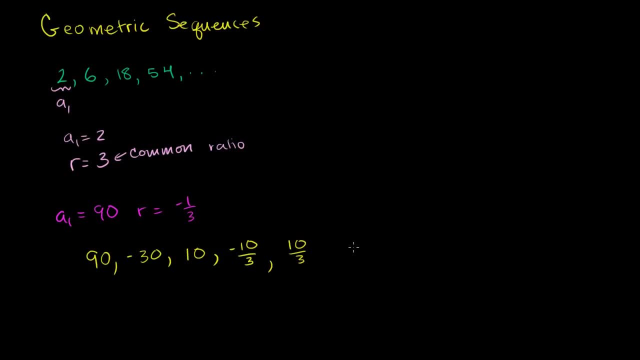 And you could just keep going on with this sequence. So that's what people talk about when they mean a geometric sequence, And I want to make one little distinction here. This always used to confuse me, because the terms are used very often in the same context. 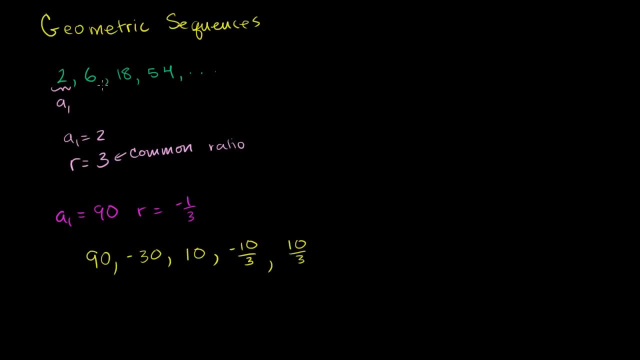 These are sequences, These are kind of a progression of numbers: 2, then 6, then 18,, 90, then negative 30, then 10, then negative 10 over 3.. Then this is positive: 10 over 9, right. 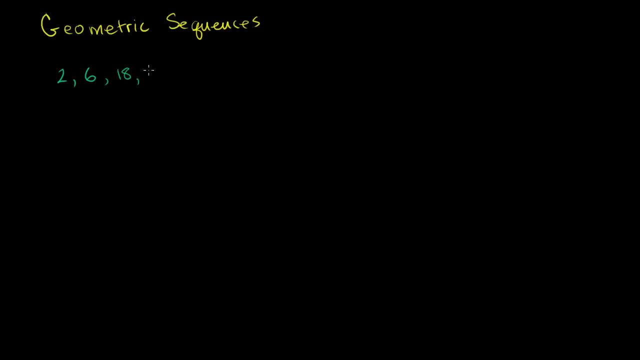 And then I multiply 18 times the number 3, and I get 54. And I just keep going that way. So I just keep multiplying by the number 3.. So I started- if we want to get some notation here- this: 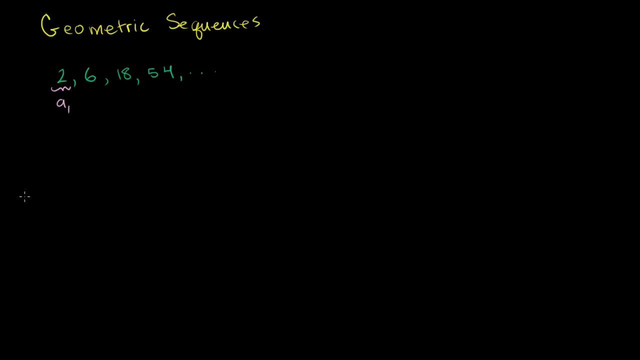 is my first term, We'll call it a1 for my sequence, And each time I'm multiplying it by a common number, And that number is often called the common ratio. So in this case, a1 is equal to 2.. 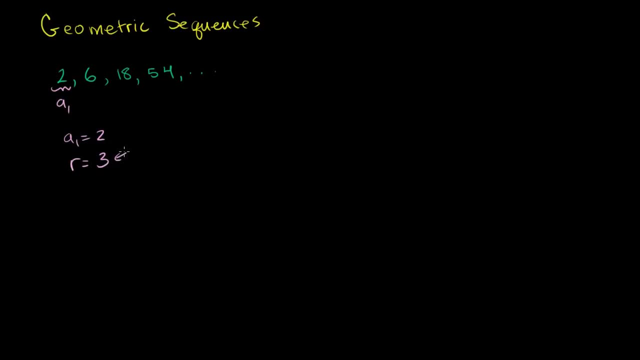 And my common ratio is equal to 3.. Common ratio. So if someone were to tell you: hey, you've got a geometric sequence, a1 is equal to 90, and your common ratio is equal to negative 3.. OK, 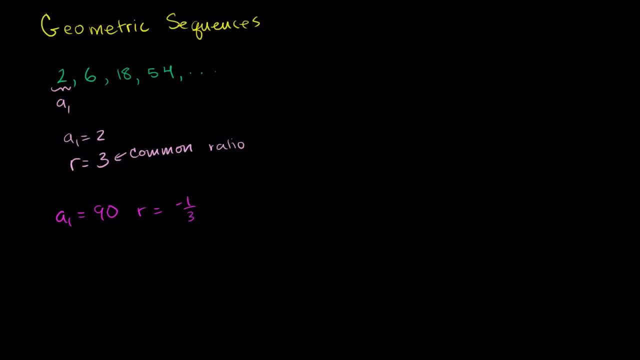 Negative 1 third. That means that the first term of your sequence is 90.. The second term is negative 1 third times 90, which is what That's: negative 30.. 1 third times 90 is 30. And then you put the negative number. 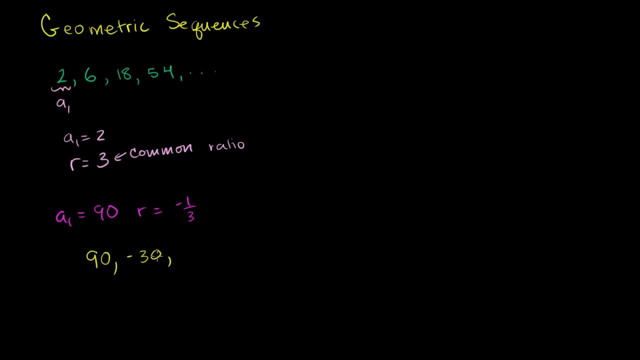 Then the next number is going to be 1 third times this. So 1 third or negative, 1 third times this. 1 third times 30 is 10.. The negatives cancel out, So you get positive, Positive, 10.. 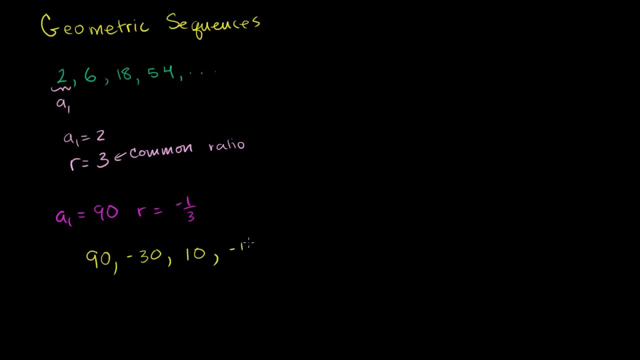 Then the next number is going to be 10 times negative: 1 third, or negative 10 thirds. And then the next number is going to be negative 10 thirds times negative: 1 third. So it's going to be positive 10 thirds. 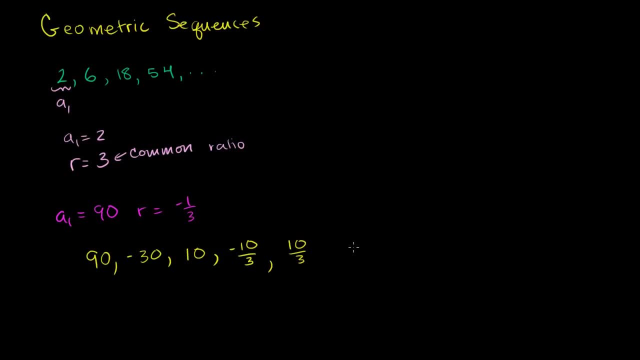 And you could just keep going on with this sequence. So that's what people talk about when they mean a geometric sequence, And I want to make one little distinction here. This always used to confuse me, because the terms are used very often in the same context. 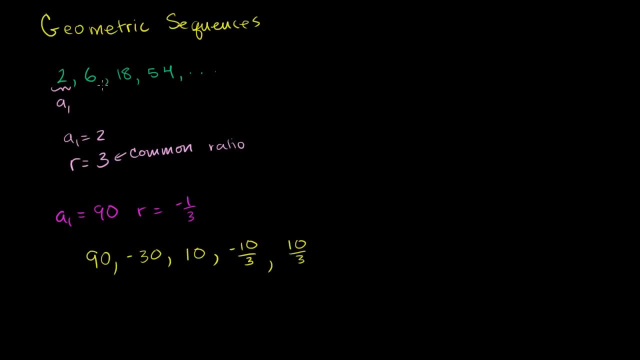 These are sequences, These are kind of a progression of numbers: 2, then 6, then 18,, 90, then negative 30, then 10, then negative 10 over 3.. Then this is positive: 10 over 9, right. 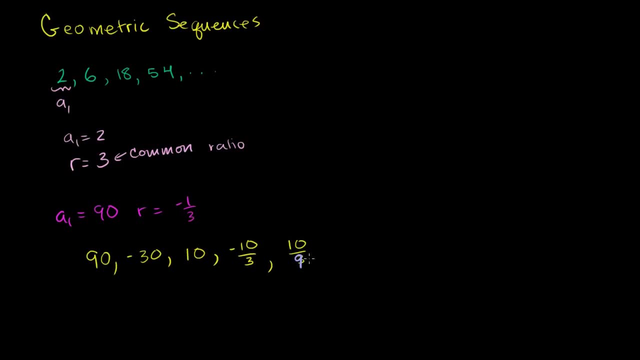 Negative: 1 third times. negative: 10 over 3. Negatives cancel out Right: 10 over 9.. Don't want to make a mistake here. These are sequences. You might also see the word a series And you might even see a geometric. 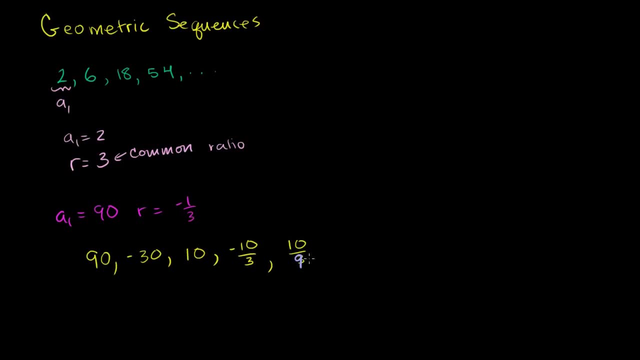 Negative: 1 third times. negative: 10 over 3. Negatives cancel out Right: 10 over 9.. Don't want to make a mistake here. These are sequences. You might also see the word a series And you might even see a geometric. 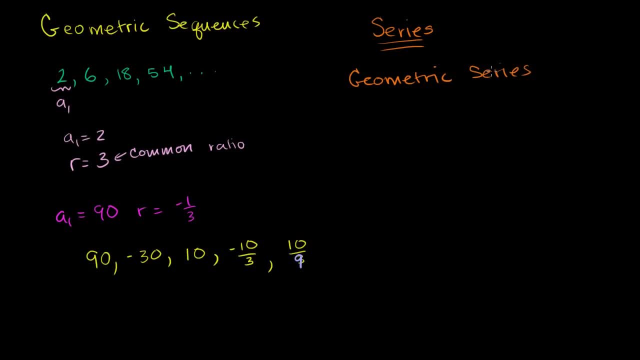 A series. the most conventional use of the word series means a sum of a sequence. So, for example, this is a geometric sequence. A geometric series would be 90 plus negative, 30 plus 10 plus negative, 10 over 3 plus 10 over 9.. 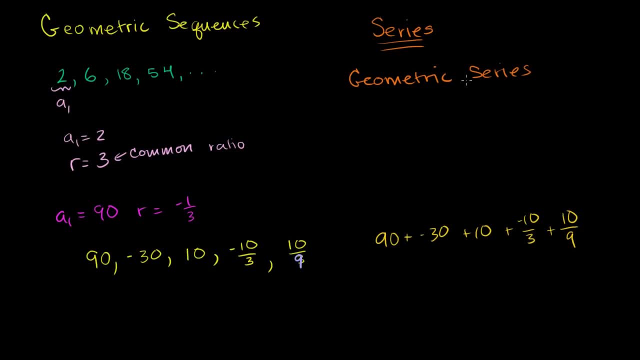 So a general way to view it is that a series is the sum of a sequence. I just want to make that clear because that used to confuse me a lot when I first learned about these things. But anyway, let's go back to the notion of a geometric 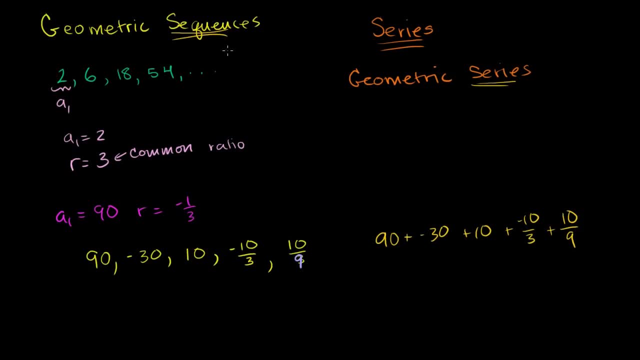 sequence and actually do a word problem that deals with one of these. So they're telling us that Ann goes bungee jumping off of a bridge above water, So Ann bungee jumping. Ann is bungee jumping On the initial jump. the cord stretches by 120 feet. 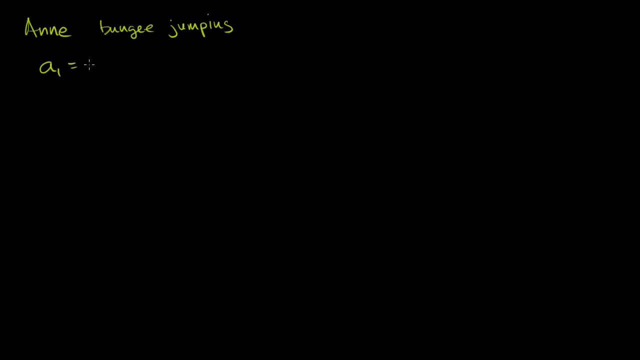 So on A1, our initial jump, the cord stretches by 120 feet. We could write it this way: We could write jump and then how much the cord stretches. So on the first, on the initial jump, on jump one, the cord stretches 120 feet. 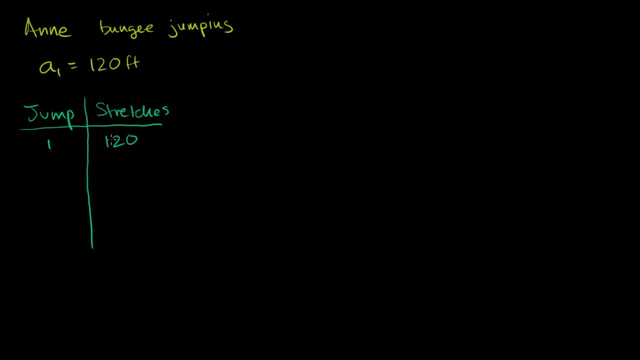 Then it says on the next bounce the stretch is 60% of the original jump, And then each additional bounce stretches the rope 60% of the previous stretch. So here the common ratio where each successive term in our sequence is going to be 60% of the previous term, or it's. 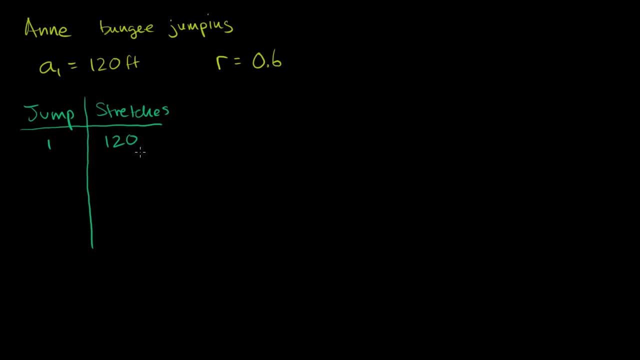 going to be 0.6 times the previous term. So on the second jump we're going to stretch 60% of that, or 0.6 times 120, which is equal to what? That's equal to 72.. 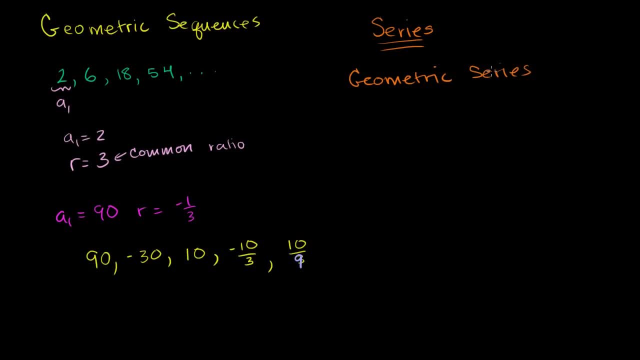 A series. the most conventional use of the word series means a sum of a sequence. So, for example, this is a geometric sequence. A geometric series would be 90 plus negative, 30 plus 10 plus negative, 10 over 3 plus 10 over 9.. 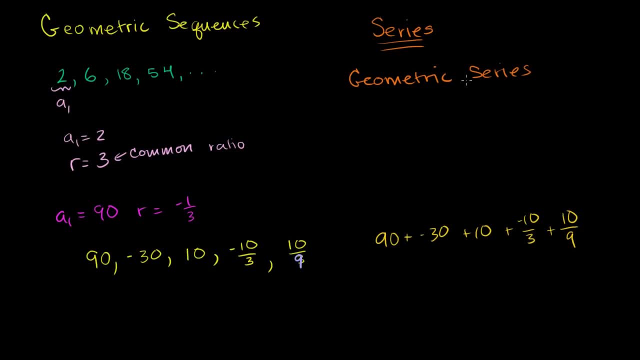 So a general way to view it is that a series is the sum of a sequence. I just want to make that clear because that used to confuse me a lot when I first learned about these things. But anyway, let's go back to the notion of a geometric 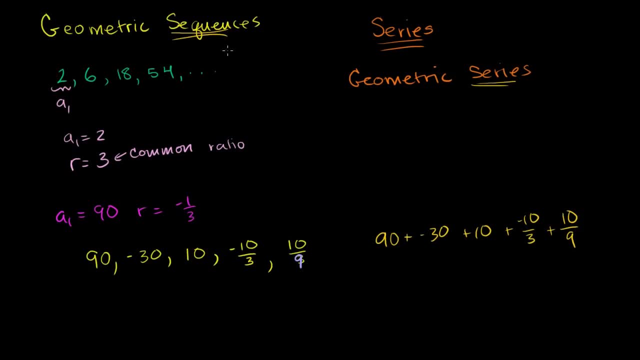 sequence and actually do a word problem that deals with one of these. So they're telling us that Ann goes bungee jumping off of a bridge above water, So Ann bungee jumping. Ann is bungee jumping On the initial jump. the cord stretches by 120 feet. 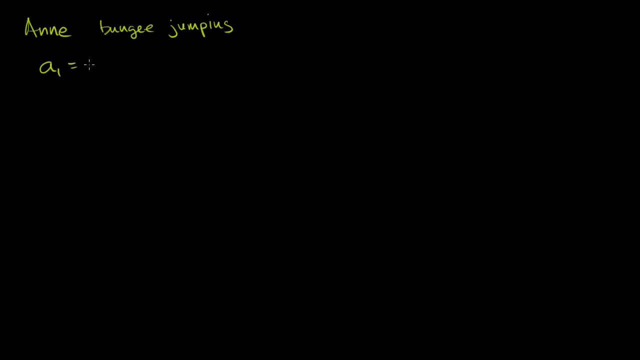 So on A1, our initial jump, the cord stretches by 120 feet. We could write it this way: We could write jump and then how much the cord stretches. So on the first, on the initial jump, on jump one, the cord stretches 120 feet. 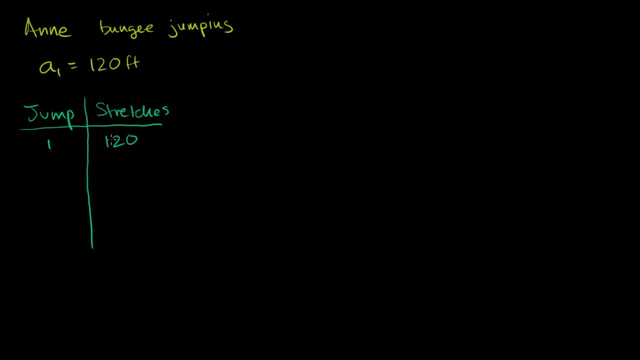 Then it says on the next bounce the stretch is 60% of the original jump, and then each additional bounce stretches the rope 60% of the previous stretch. So here the common ratio where each successive term in our sequence is going to be 60% of the previous term, or it's. 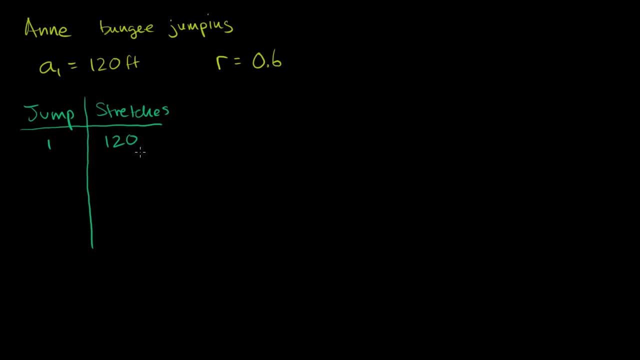 going to be 0.6 times the previous term. So on the second jump we're going to stretch 60% of that, or 0.6 times 120, which is equal to what? That's equal to 72.. 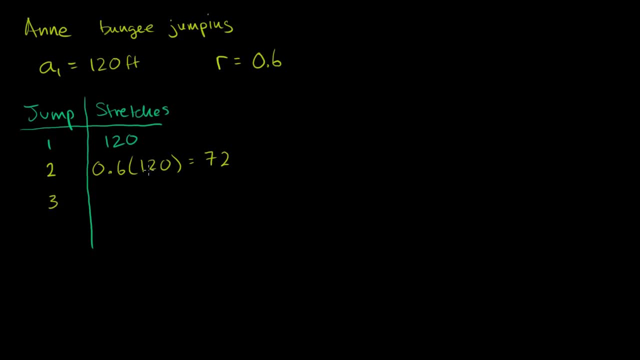 Then on the third jump, we're going to stretch 0.6 of 72, or 0.6 times this, So it would be 0.6 times 0.6 times 120.. And then on the fourth jump- notice over here. 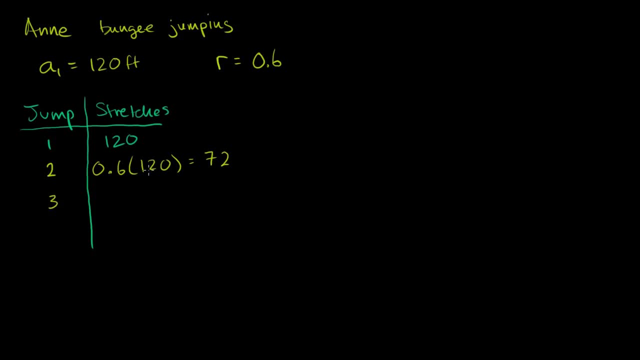 Then on the third jump, we're going to stretch 0.6 of 72, or 0.6 times this, So it would be 0.6 times 0.6 times 120.. And then on the fourth jump- notice over here. so on the 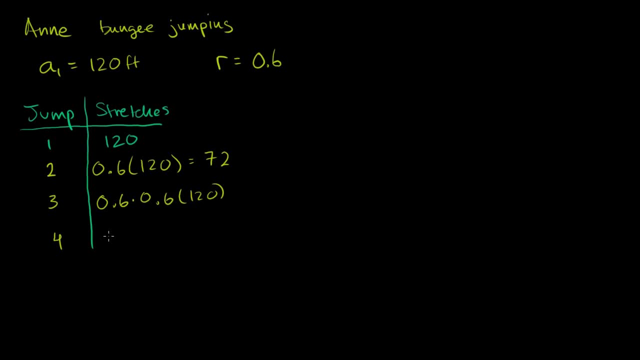 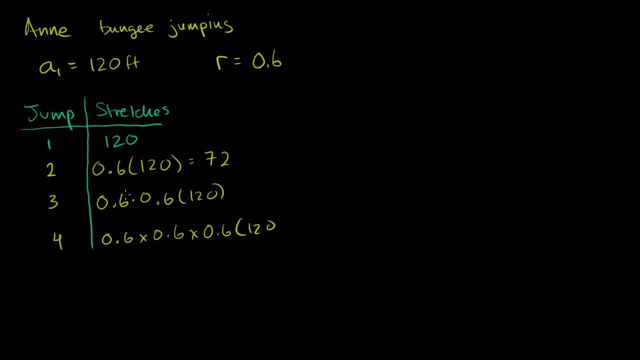 60% of this jump. So every time we're 60% of the previous jump. So if we wanted to make a general formula for this, just based on the way we've defined it right here- so the stretch on the nth jump- what would it be? 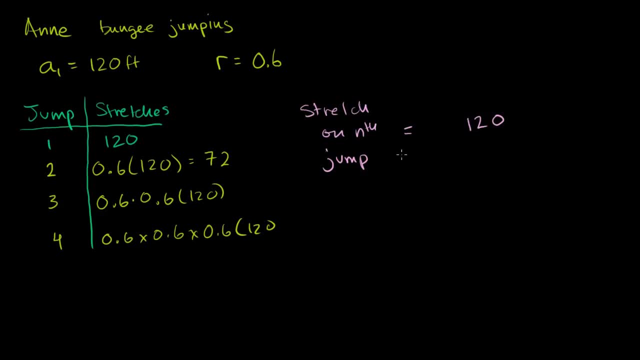 So let's see, We start at 120.. And 120 times 0.6.. Let me do the 0.6 here: Times 0.6 to the what, To the n minus 1.. Now, how did I get this? 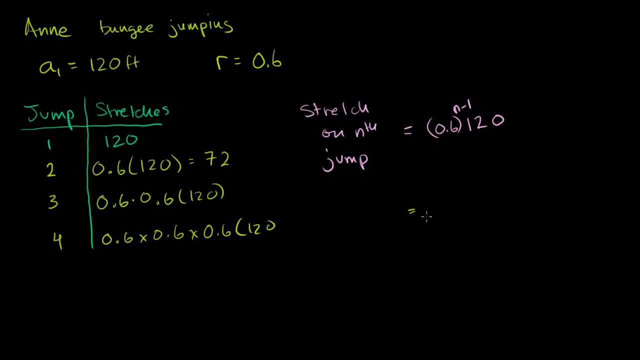 Let me write this a little bit neater. So this is equal to 0.6.. Actually, let me write the 120 first. This is equal to 120 times 0.6.. To the n minus 1.. How did I get that? 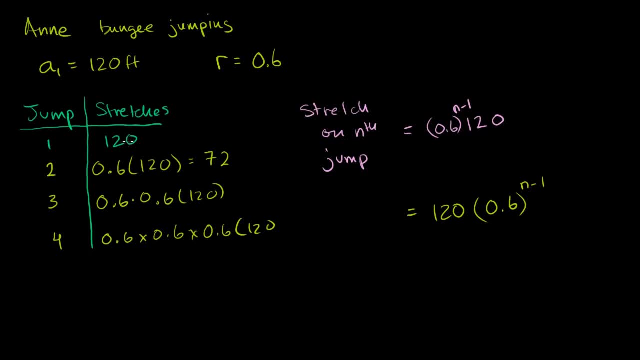 Well, we're defining the first jump as stretching 120 feet. So when you put n is equal to 1. here you get 1 minus 1. 0.. So you have 0.6 to the 0th power. 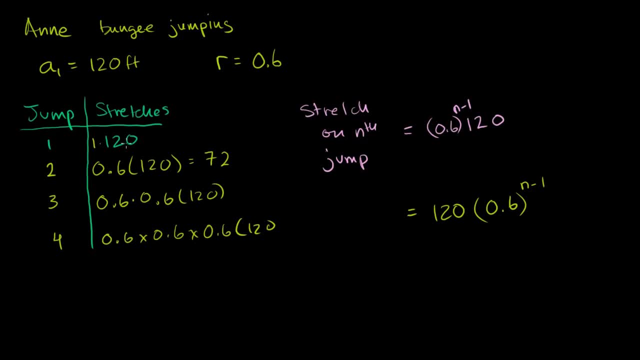 So you just get a 1 here, And that's exactly what happened on the first jump. Then on the second jump you put a 2 minus 1.. And notice: 2 minus 1 is the first power And we have exactly 1.6 here. So I figured it was n minus 1, because when n is 2, we have 1.5.. So you get 0.6 to the 0.6 here And notice, 2 minus 1 is the first power. 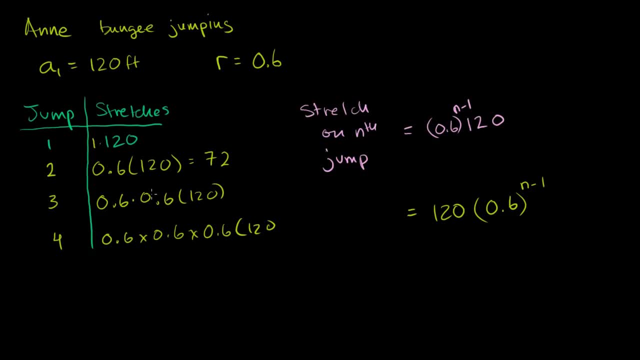 And we have exactly 1.6 here. So I figured it was n minus 1, because when n is 2, we have 1.6.. have 1.6.. When n is 3, we have 2.6's multiplied by themselves. 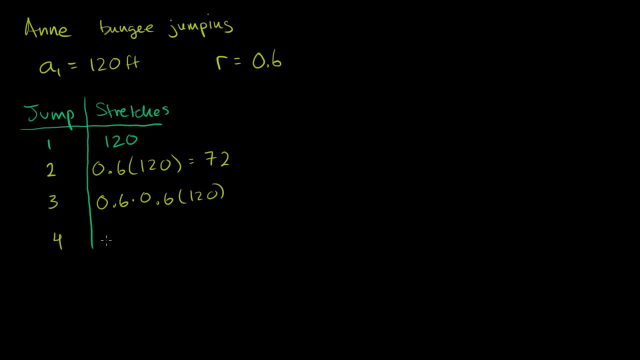 So on the fourth jump we're going to have 0.6 times 120.. times 0.6 times 0.6 times 120.. 60% of this jump. So every time we're 60% of the previous jump. 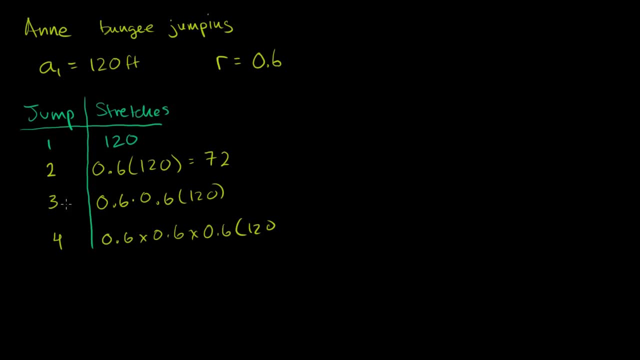 So if we wanted to make a general formula for this, just based on the way we've defined it right here- so the stretch on the nth jump, what would it be? So let's see, we start at 120 times 0.6.. 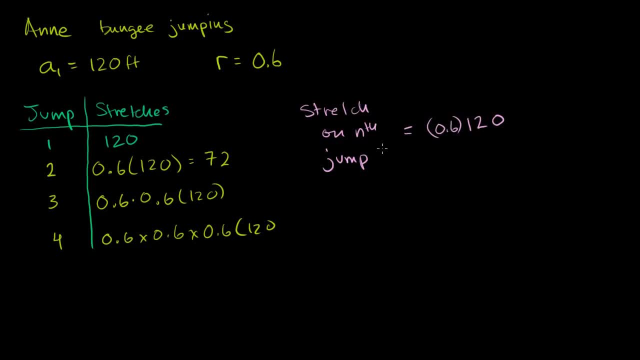 Let me do the 0.6 here. Times 0.6 to the what To the n minus 1.. Now, how did I get this? Let me write this a little bit neater. So this is equal to 0.6.. 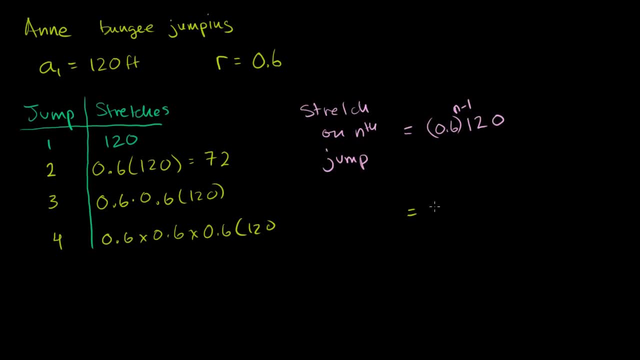 Actually, let me write the 120 first. This is equal to 120 times 0.6.. 0.6 to the n minus 1.. How did I get that? Well, we're defining the first jump as stretching 120 feet. 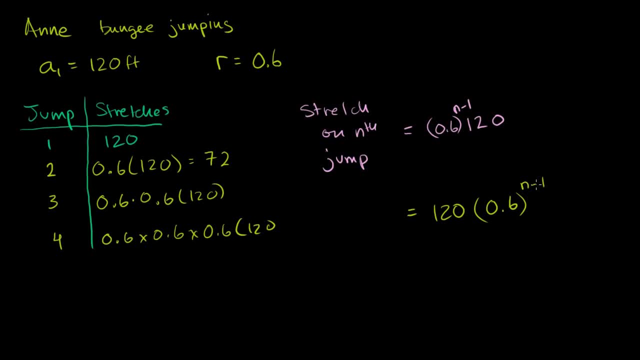 So when you put n is equal to 1, here you get 1 minus 1, 0.. So you have 0.6 to the 0th power. So you just get a 1 here, And that's exactly what happened on the first jump. 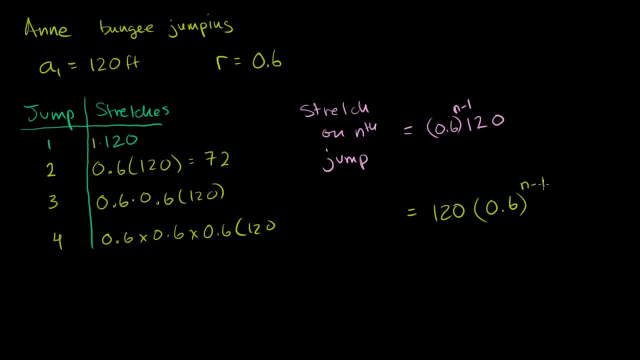 Then on the second jump you put a 2 minus 1.. And notice: 2 minus 1 is the first power And we have exactly 1.6 here. So I figured it was n minus 1.. Because when n is 2, we have 1.6. 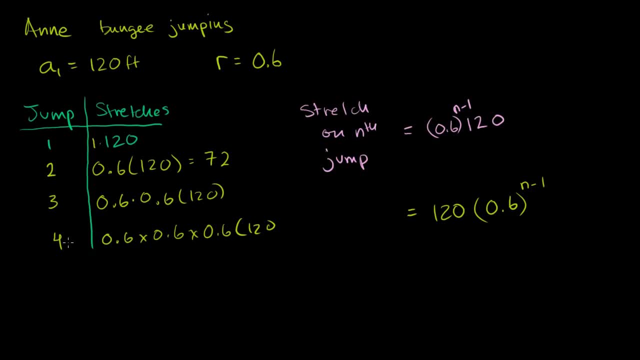 When n is 3, we have 2.6's multiplied by themselves. When n is 4, we have 0.6 to the third power. So, whatever n is, we're taking 0.6 to the n minus 1th power. 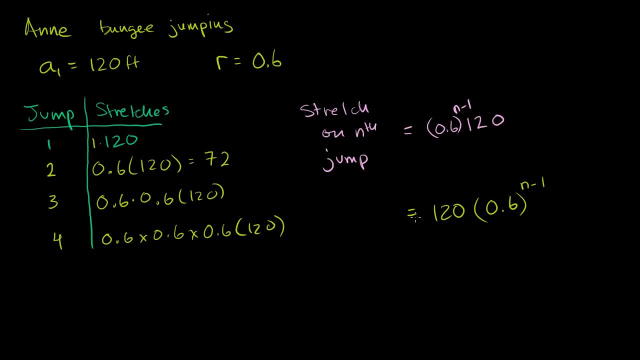 And of course we're multiplying that times 120.. Now in the question they also ask us what will be the rope stretch on the 12th bounce. On the 12th bounce And overheating. So over here I'm going to use the calculator. 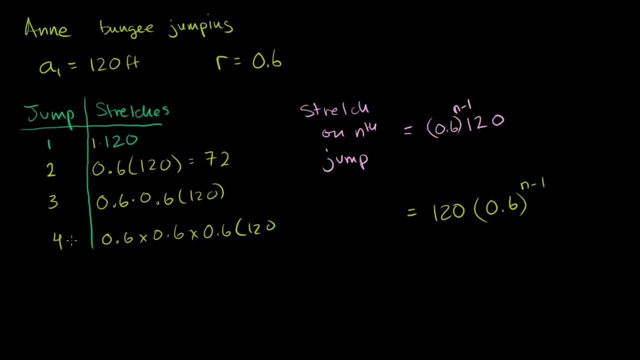 When n is 4, we have 0.6 to the third power. So, whatever n is, we're taking 0.6 to the n minus 1th power And of course we're multiplying that times 120.. Now in the question they also ask us what will be the rope? 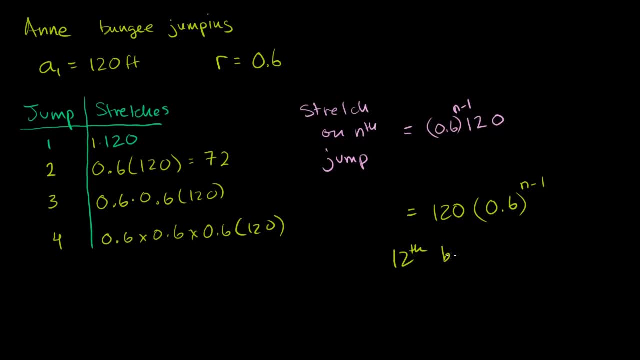 stretch on the 12th bounce, On the 12th bounce And over here I'm going to use the calculator And actually let me correct this a little bit. This isn't incorrect, but they're talking about the bounce. 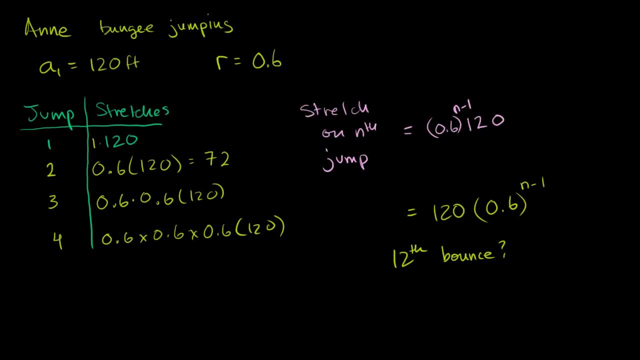 And we could call the jump the 0th bounce. So let me change that. This isn't wrong, but I want to make it a little bit more. I think this is where they're going with the problem. So you can view the initial stretch as the 0th bounce. 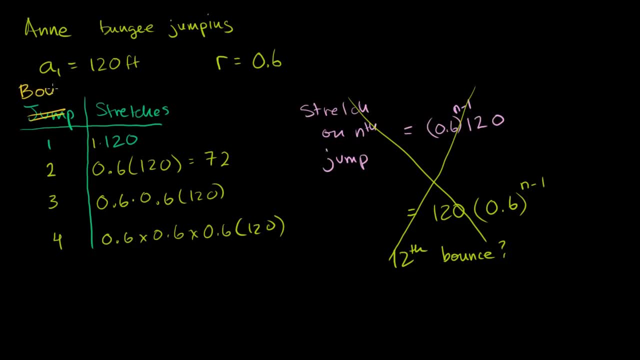 So let me, Instead of labeling it jump, let me label it bounce. So the initial stretch is the 0th bounce, Then this would be the first bounce, the second bounce, the third bounce, And then our formula becomes a lot simpler. 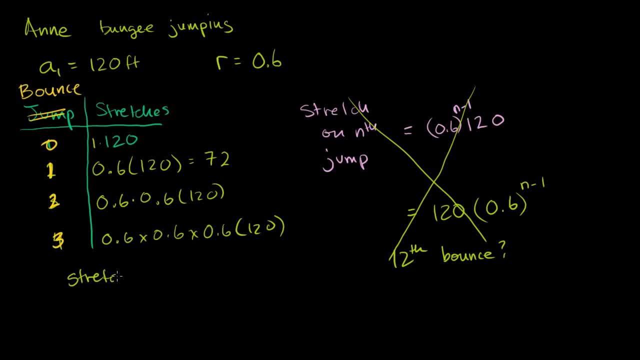 Because if you said the stretch on nth bounce then the formula just becomes 0.6 to the n, That's 1 times 120, right On the 0th bounce- that was our original stretch- You get 0.6 to the 0.. 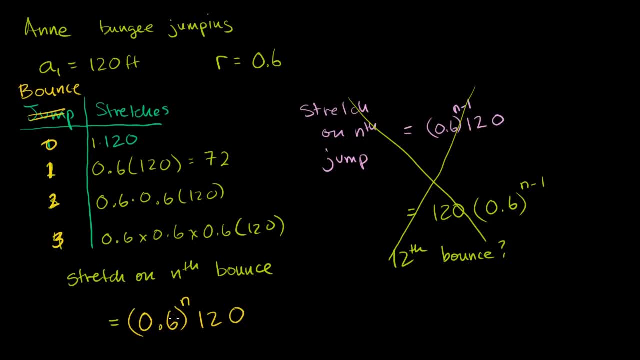 That's 1 times 120.. On the first bounce, 0.6 to the 1. You have 1.6 right here, 0.6 times the previous stretch or the previous bounce. So this has it in terms of bounces. 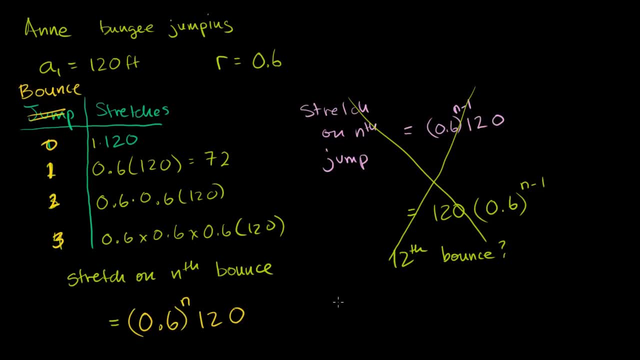 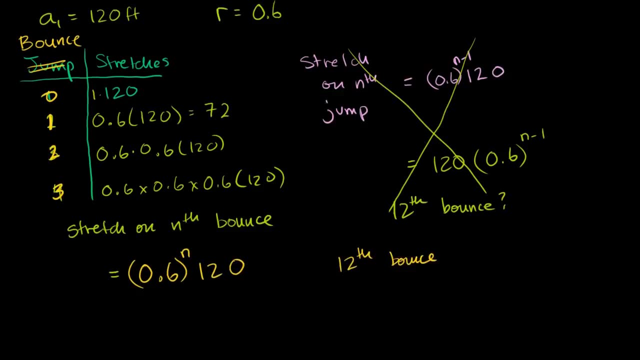 which I think is what the questioner wants us to do. So what about the 12th bounce? 12th bounce Using this convention right, This convention right there. So if we do the 12th bounce, let's just. 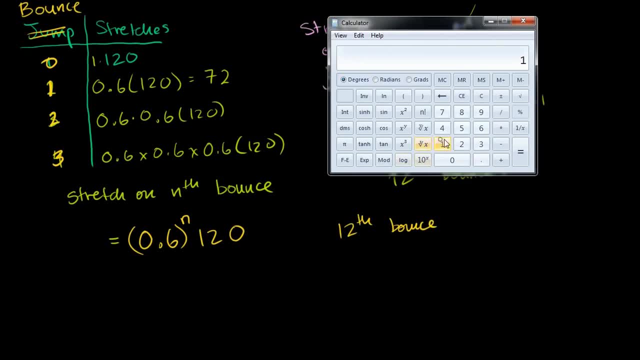 get our calculator out. We're going to have 120 times 0.6 to the 12th power And hopefully we'll get order of operations right, Because exponents take precedence over multiplication, So it'll just take the 0.6 to the 12th power only. 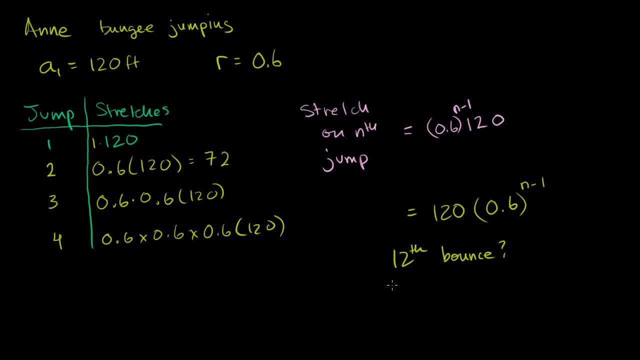 And actually let me correct this a little bit. This isn't incorrect, but they're talking about the bounce And we could call the jump the 0th bounce. So let me change that. This isn't wrong, but I want to make it a little bit more. I. 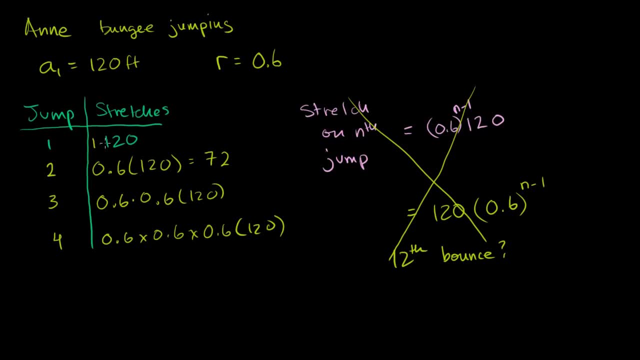 think this is where they're going with the problem. So you can view the initial stretch as the 0th bounce. So let me, instead of labeling it jump, let me label it bounce. So the initial stretch is the 0th bounce. 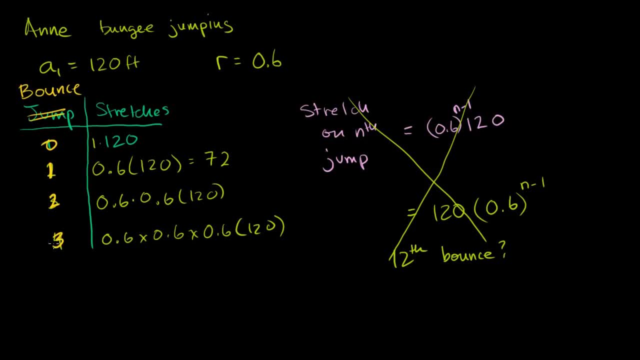 Then this would be the first bounce, the second bounce, the third bounce And then our formula becomes a lot simpler, Because if you said the stretch on nth bounce, then the formula just becomes 0.6 to the n times 1.2.. 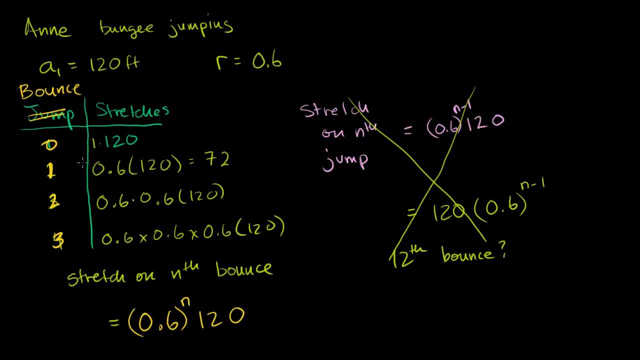 0.6 to the n times 1.2.. 0.6.. 120, right On the 0-th bounce. that was our original stretch. you get 0.6 to the 0,, that's 1 times 120.. 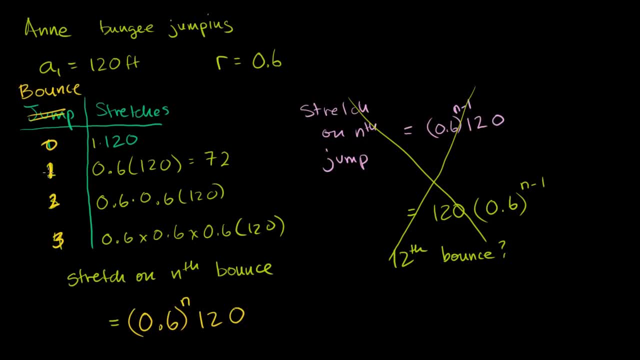 On the first bounce, 0.6 to the 1,, you have 1.6 right here, 0.6 times the previous stretch or the previous bounce. So this has it in terms of bounces, which I think is what. 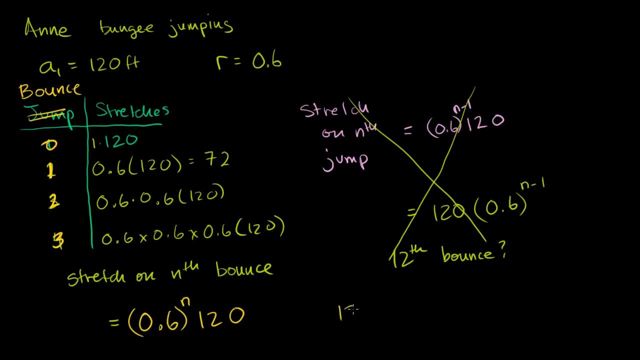 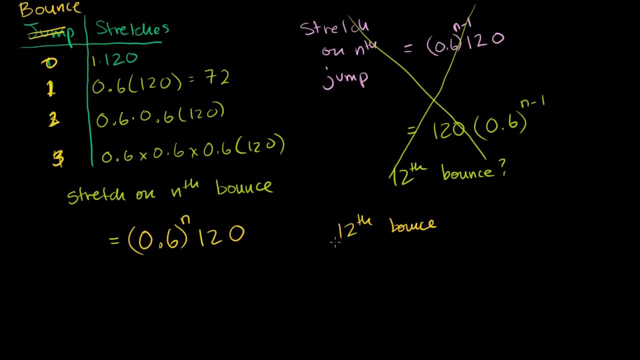 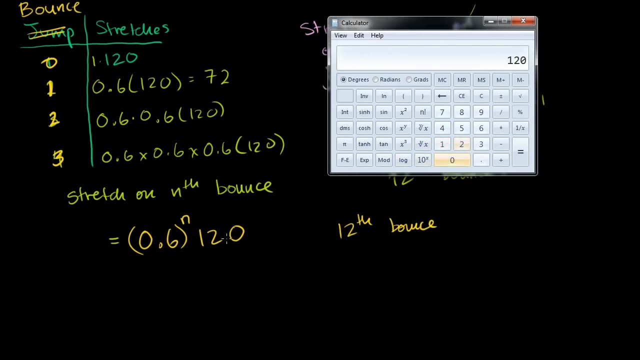 the questioner wants us to do. So what about the 12-th bounce? 12-th bounce using this convention, right there. So if we do the 12-th bounce, let's just get our calculator out. we're going to have 120 times 0.6 to the 12-th power. 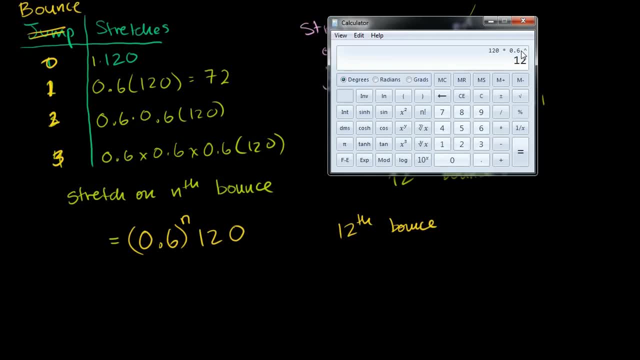 And hopefully we'll get order of operations right, because exponents take precedence over multiplication, so it'll just take the 0.6 to the 12-th power only, And so this is. So this is equal to 0.26 feet. 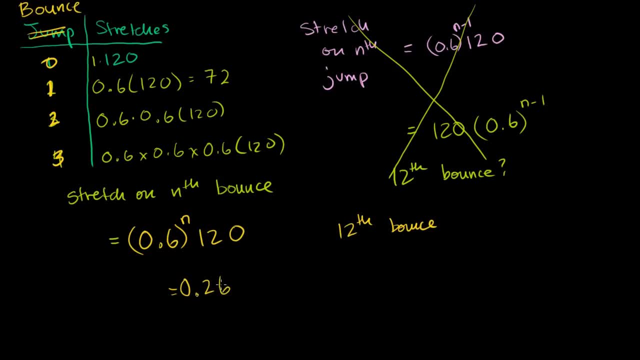 So after your 12-th bounce she's going to be barely moving. She's going to be moving about 3 inches on that 12-th bounce. Well, anyway, hopefully you found this helpful and I apologize for the slight divergence here.